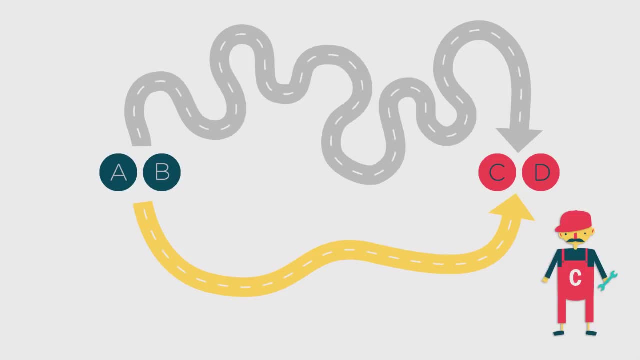 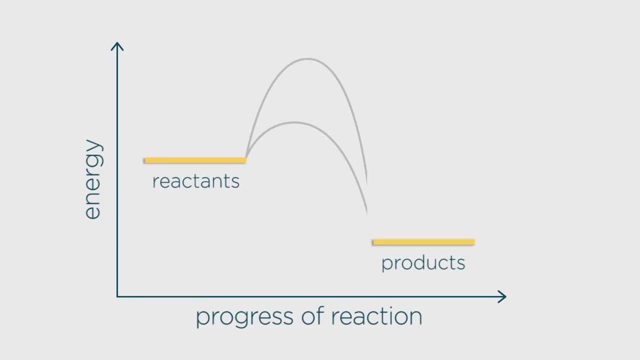 for the reaction to occur. This alternative pathway has a lower activation energy than the pathway without the catalyst. Here are the two pathways for a reaction: The blue pathway is the energy profile for the reaction without the catalyst and the red pathway is the energy profile for the reaction with the catalyst. You can see here that with the 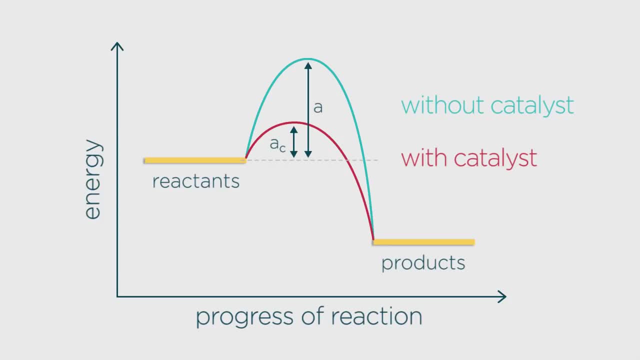 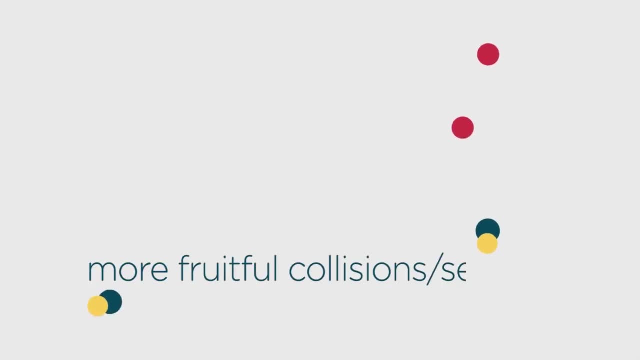 catalyst, the activation energy is lower. As a result of the activation energy being lower, there are more molecules with the required activation energy and so more fruitful collisions occur and hence the reaction is faster. Do you know where catalysts are used in everyday? 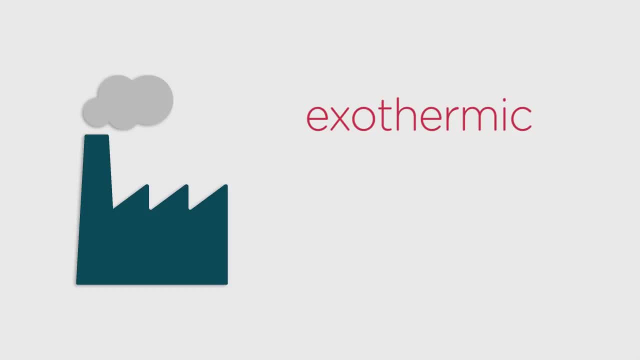 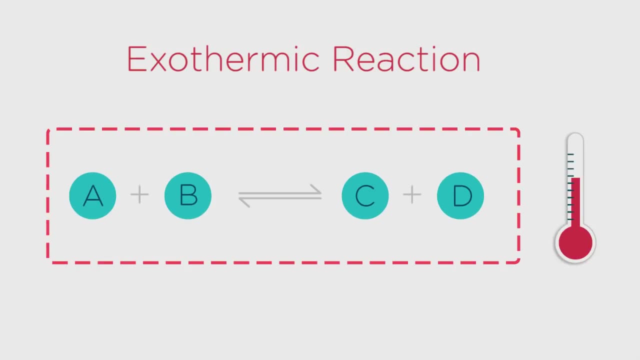 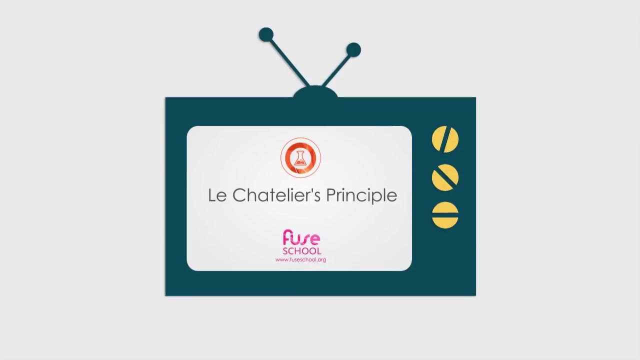 life. Most manufacturing processes are exothermic for economic reasons. The heat given out is used to maintain the operating temperature of the reaction. Exothermic reactions cannot run at too high temperatures as the yield will be too low. So as we cannot increase, 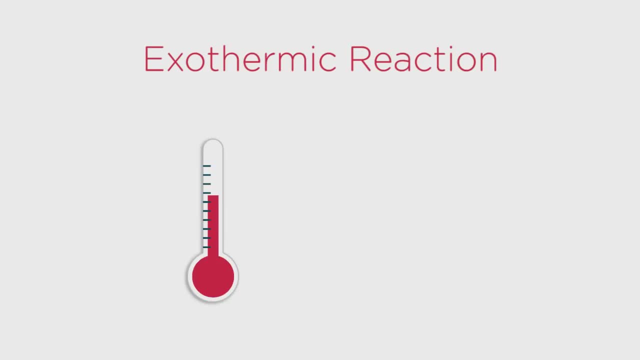 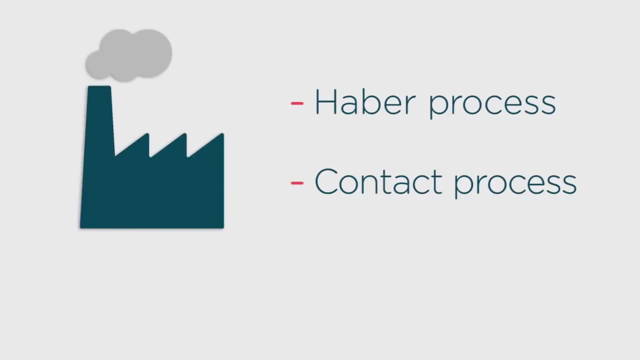 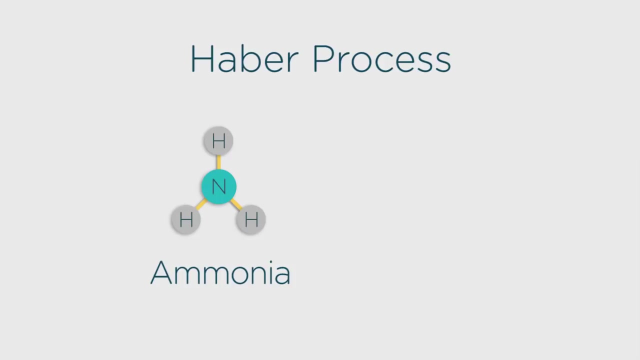 the rate of these exothermic reactions. by having an exothermic reaction, we need to use catalysts to increase the rate of reaction. Here are two manufacturing processes that use catalysts. Firstly, the harbour process to manufacture ammonia, most of which is used in fertilisers. In this process, iron is the 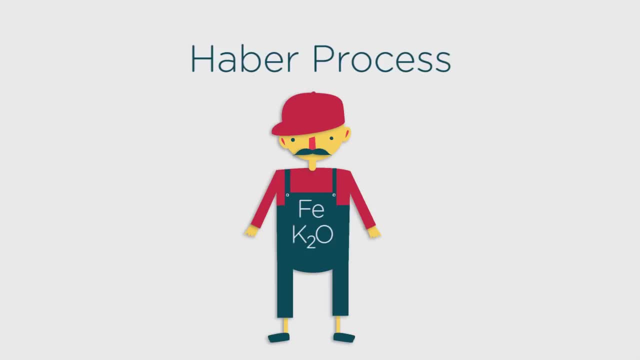 catalyst, The iron has potassium oxide, which acts as a promoter added to increase its efficiency. And secondly, the contact process to manufacture sulfuric acid. Sulfuric acid, which is used to make detergents and fertilisers, Vanadium 5 oxide sometimes. 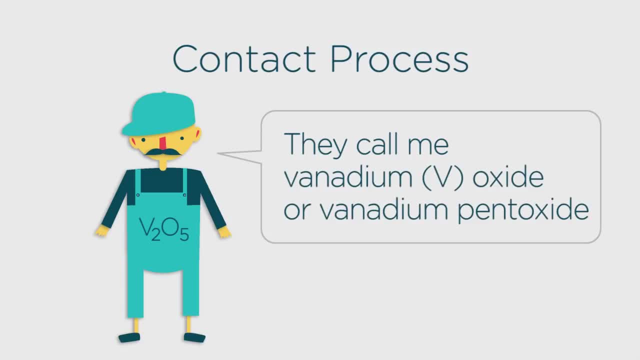 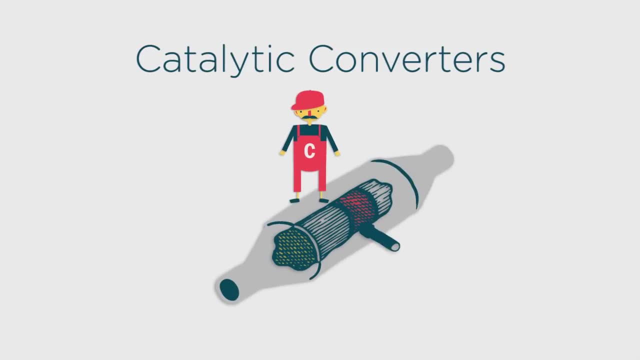 known as vanadium pentoxide, is the catalyst in the contact process. Catalysts are also used in catalytic converters in vehicles. These catalysts remove toxic exhaust gases by converting them into harmless products. So to recap, catalysts speed up chemical reactions without themselves being used up.